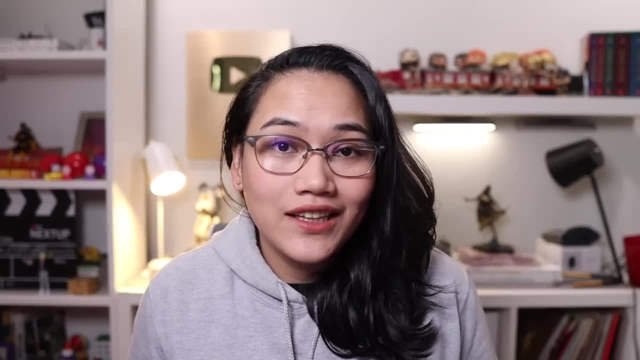 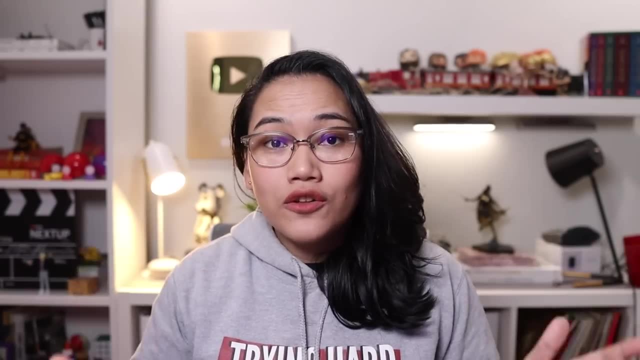 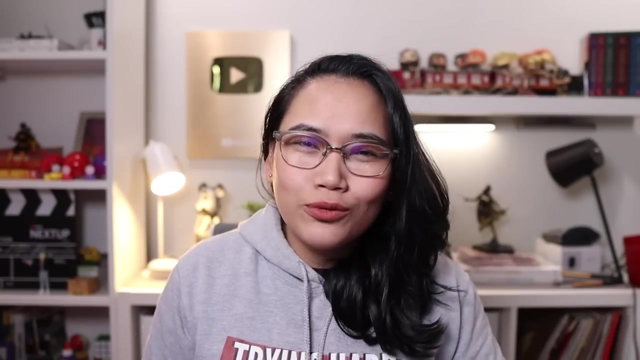 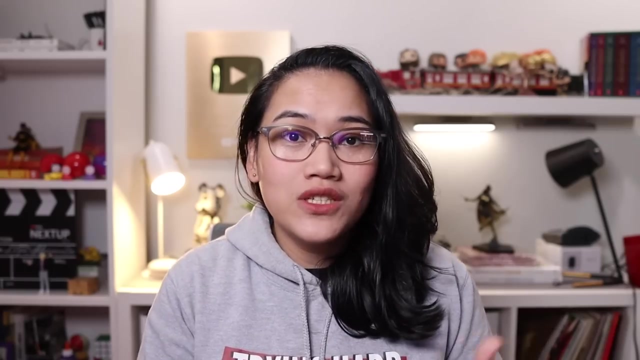 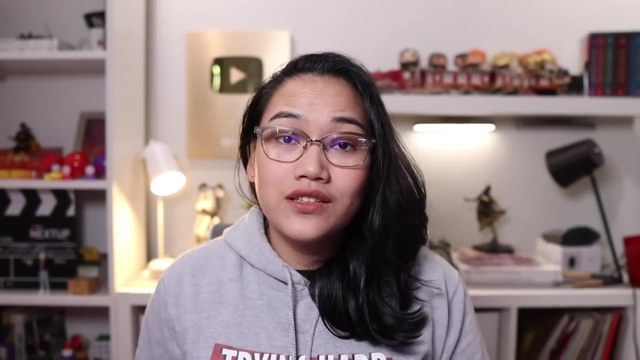 going and for me to keep creating all of the easy content. okay, now let's jump right into this. now. the first method we're going to test is just straightforward, na solving ng problem. Tinago ko muna yung options right here, kasi alam ko yung iba sa inyo pilosopo, so ang gagawin ninyo ay uunahan ninyo ako, Pero ngayon titinan lang muna natin yung problem na to, and I'm going to time myself solving this using algebra. okay, sabi ito: the sum of two numbers is 40 if twice the smaller number is five more than the bigger number. what is the smaller number? 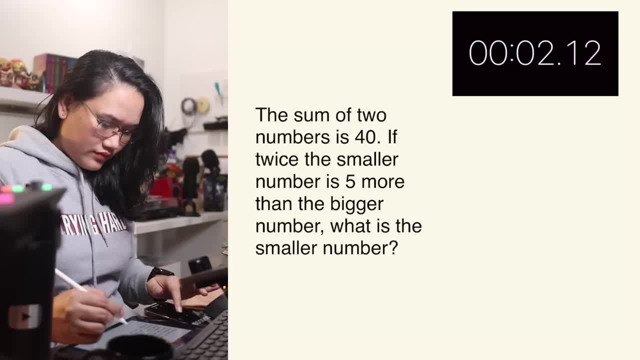 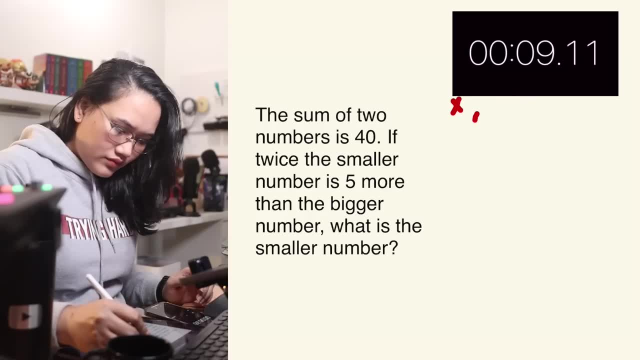 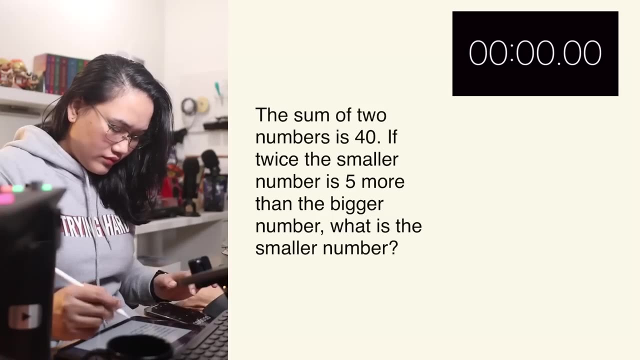 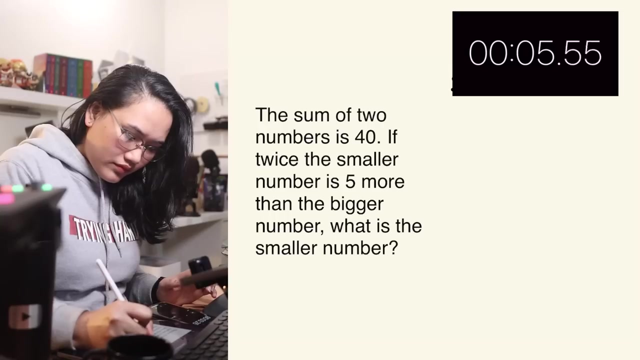 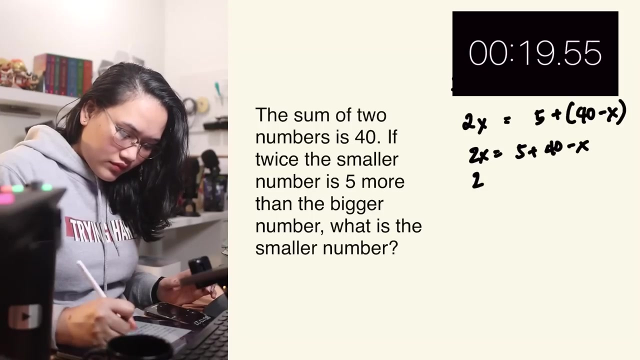 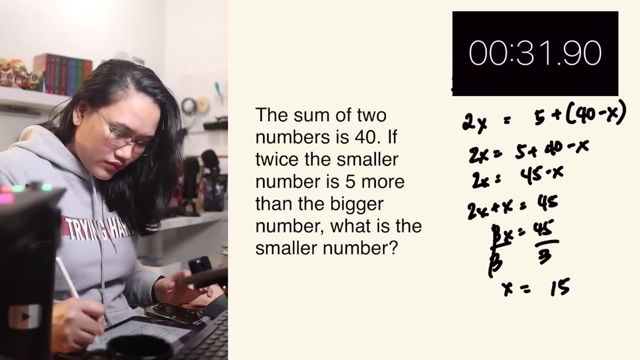 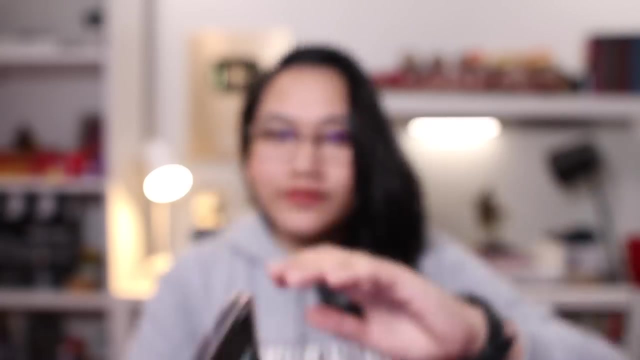 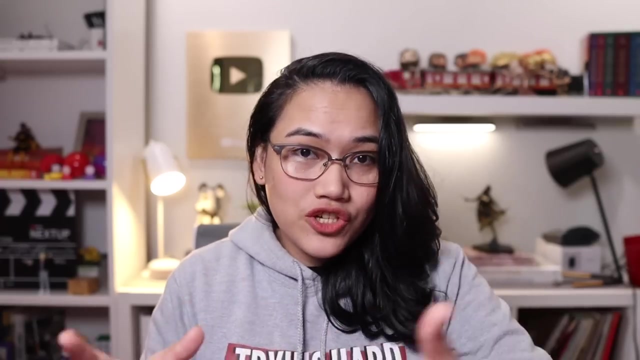 Saim na din kawan. Okay, so I finished answering the problem and it took me about 32 seconds, and And answer pa lang yan. ha, hindi pa counted yung shading doon sa mismo answer sheet. As you saw, ang ginamit kong method is yung official method, algebra. 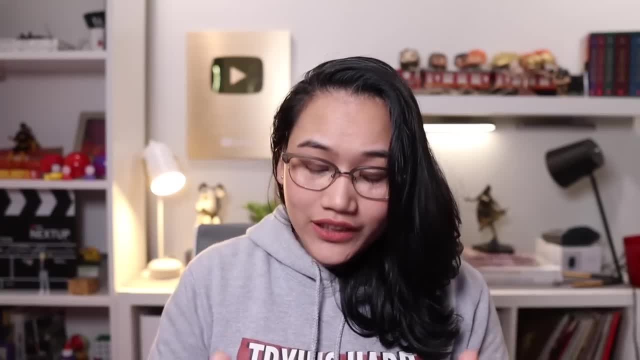 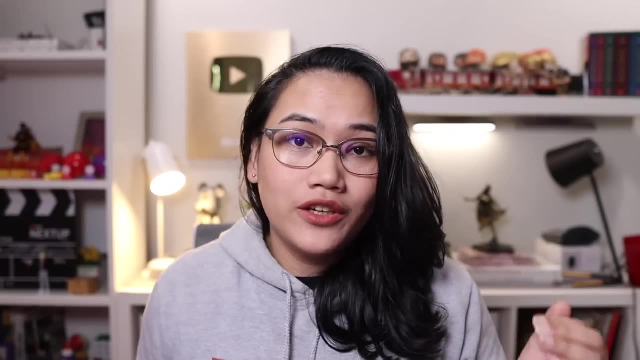 So meron tayong x, meron tayong 40 minus x, and then I converted yung problem into an equation, solved the equation and then found yung missing number, which is the smaller number. Now ang challenge sa ganitong method, lalo na pagdating sa exam, na merong time limit, 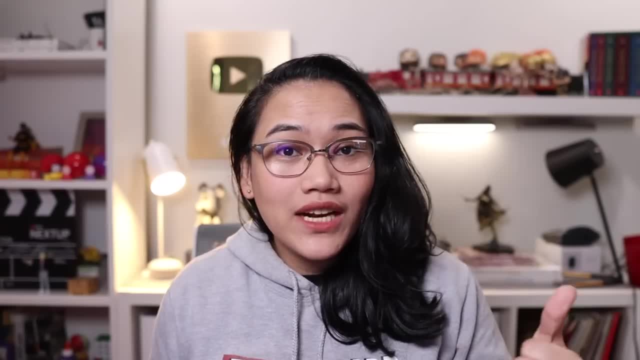 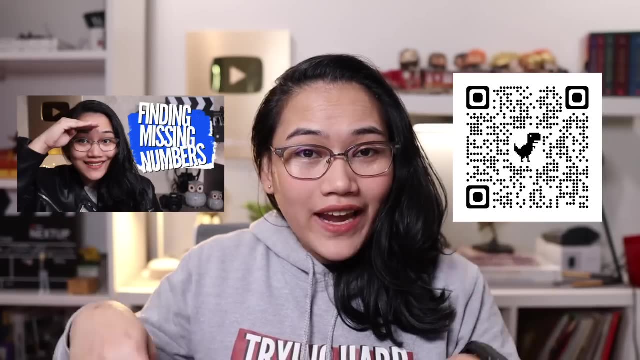 is that umuubos siya ng oras? Siyempre, una sa lahat. ang unang tanong would be: alam mo ba lahat ng mga lessons na relevant dito? Now I do have a full lesson on finding yung sagot sa ganitong klaseng tanong sa algebra ng mga missing numbers. 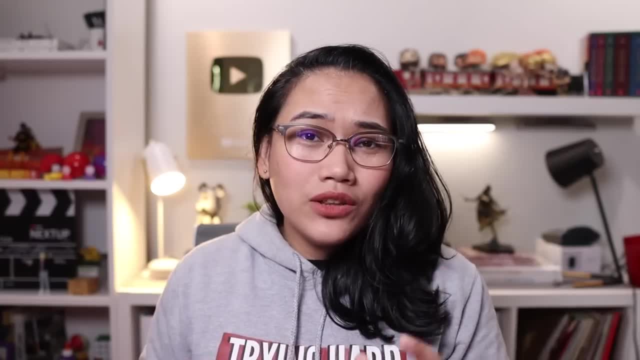 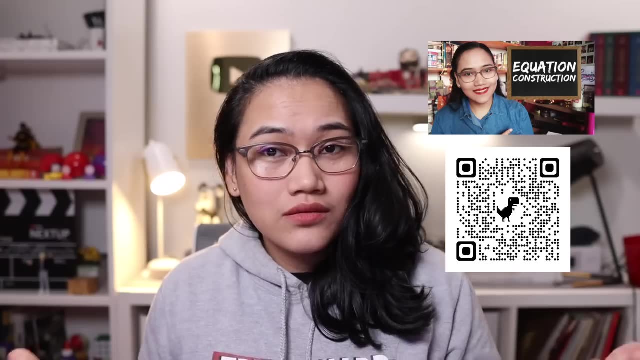 If you haven't seen those videos yet, lilay ko na lang din sa taas. Pero maliban doon sa mismo word problem type. kailangan marunong ka rin kung paano mag-translate ng sentences into equations. Again, may video din tayo niyan. 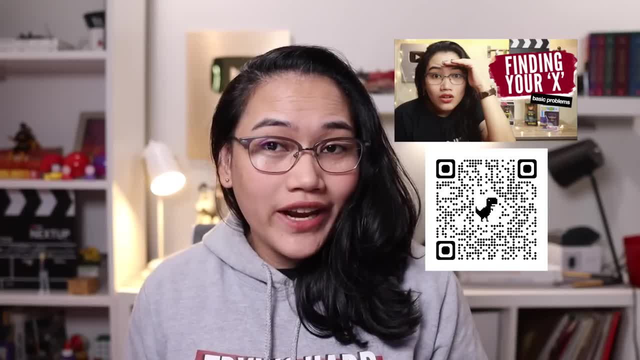 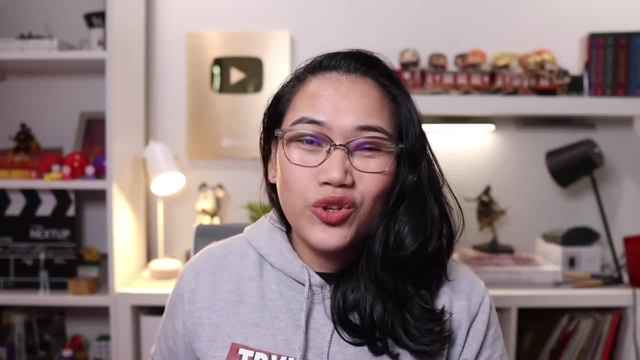 Dapat marunong ka mag-solve ng algebra or mag-solve for x Again, may series din tayo. All of these things need to work together for you to get to the correct answer. So yun yung medyo downside niya. 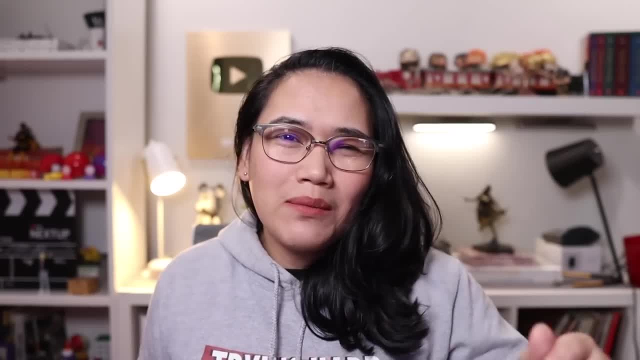 Although makukuha mo talaga yung official na sagot, kung hindi mo naman alam ang lahat ng mga components, baka hindi ka umabot doon. Now, yung next method na i-test natin is trial and error. 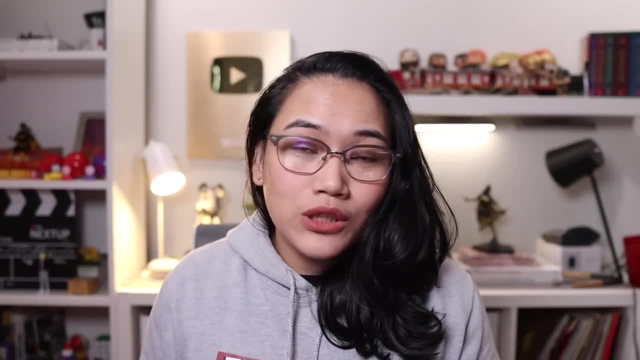 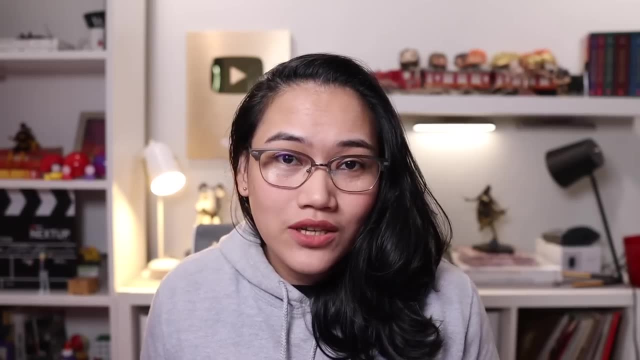 Sa totoo lang, effective ang trial and error in my opinion, Kasi nga naman sa multiple choice ng mga questions may options ka na. All you need to do is to figure out kung alin sa mga options na yan ang tamang sagot. 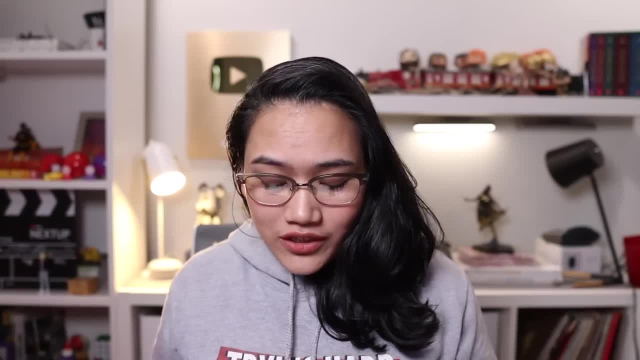 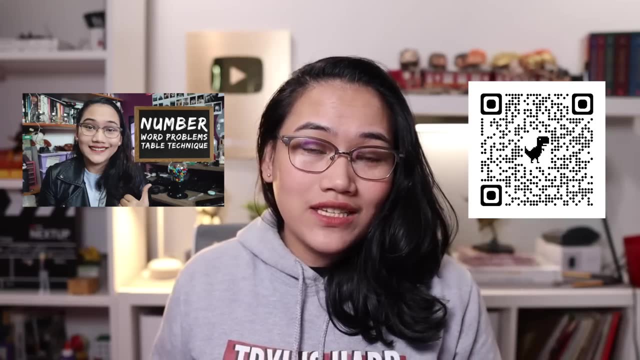 So hindi mo na kailangan i-try lahat ng numbers sa buong mundo. You just need to try yung apat na given, or even less than that. Now I'll show you how I use trial and error dito sa ganun klaseng tanong. 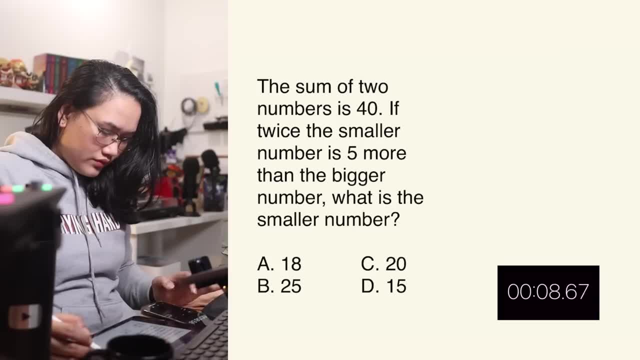 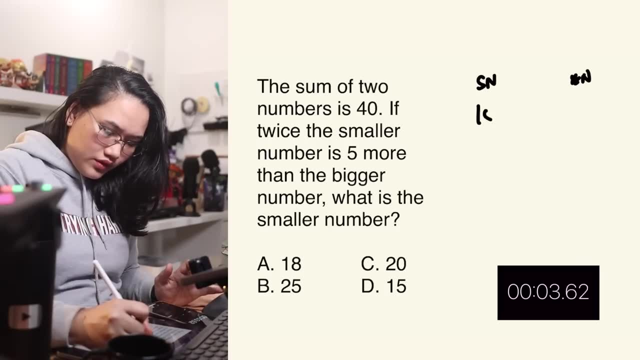 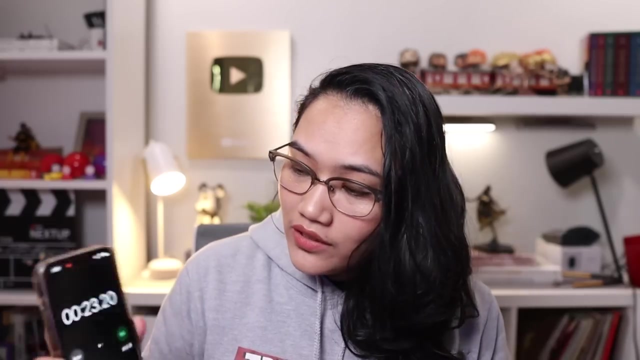 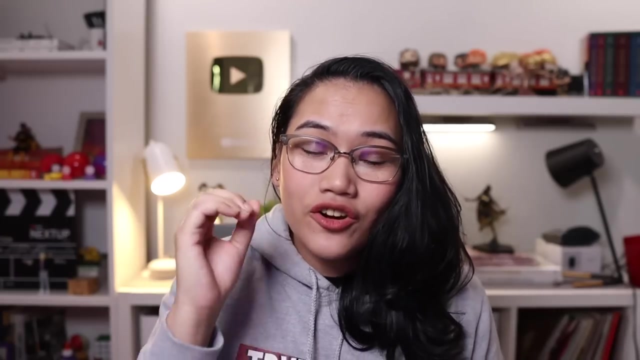 Okay, Orasan din natin. Okay. so by using trial and error I answer the question in 23 seconds. But that entire thing, yung trial and error, is banking on you knowing kung paano mo i-try kung tama yung sagot. 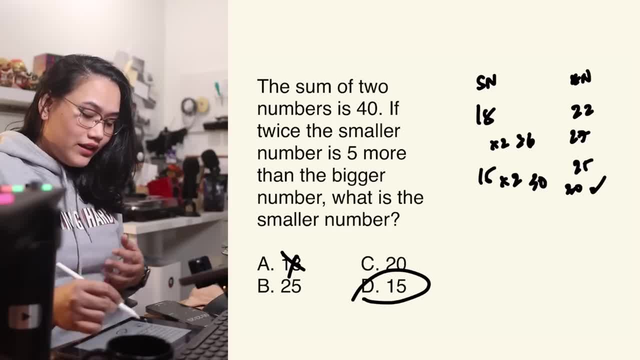 Sa case ko, ang ginawa ko, inanap ko yung bigger number na paired, Kasi sabi ang sum daw ay 40. So ang 18, ang kapatid Pares niya, ay 22.. 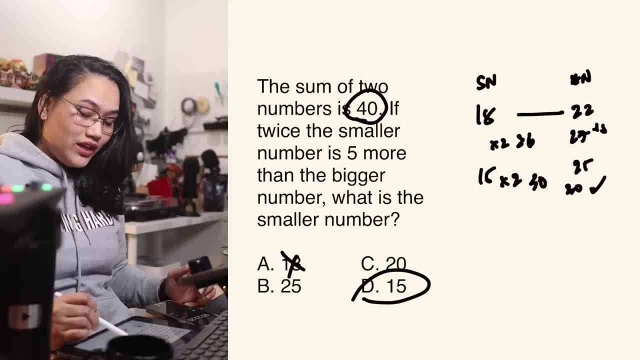 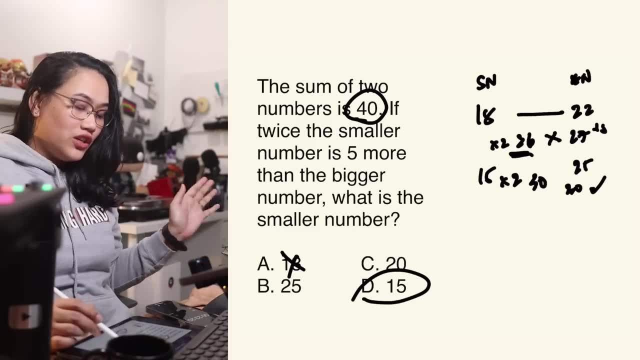 Pin-loss: 5 ko siya to get 27.. Ito yung times 2 ko yung 18.. Hindi siya equal At dahil mas mataas yung smaller number na side dito sa aking mini-equation na check ko dito. 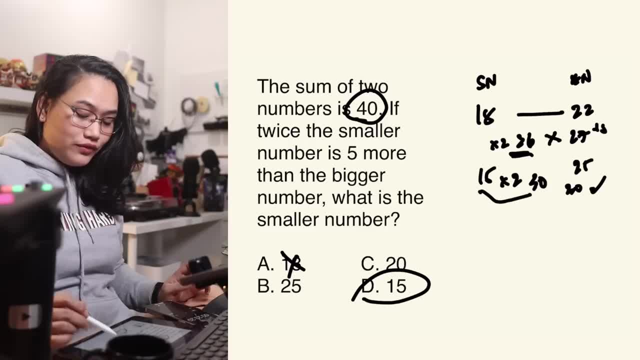 Ang kinuha ko yung 15.. To make sure na tama ito, yung times 2 ko yung 15.. Naging yung 30. Yung 25, dinagdagan ko din siya ng 5.. 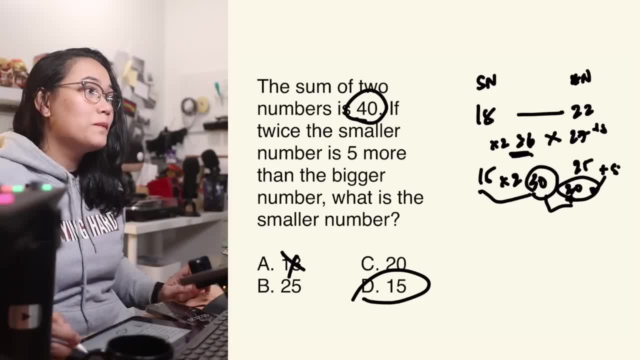 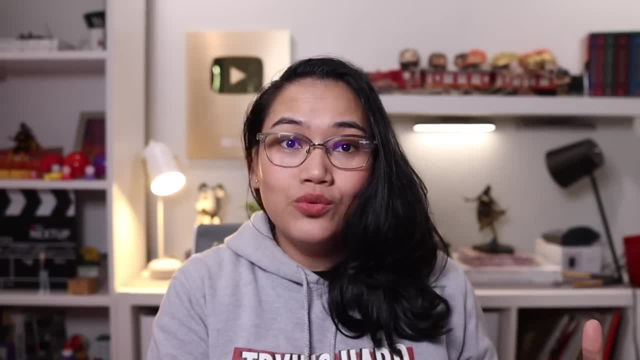 And lumabas ay 30.. Equal na sila, which means 15.. Ang sagot: If you don't understand this part right here, doon na pa pasok yung you may need to solve Using an equation, Or skip nyo na lang. 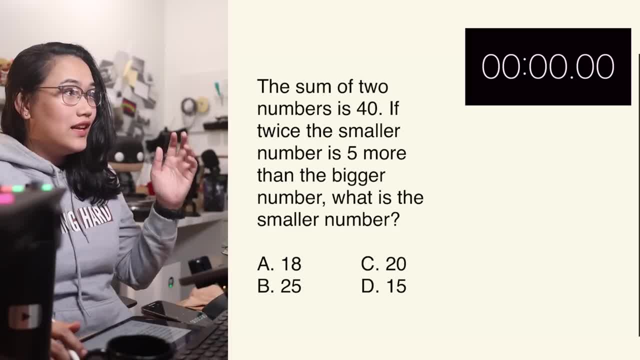 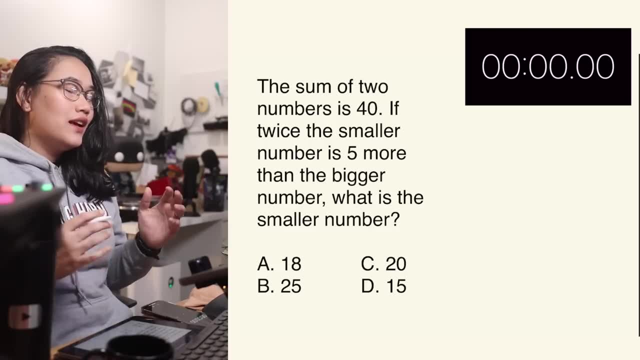 Or hulaan mo na lang. Now, yung next method na pag-uusapan natin is elimination. Sa opinion ko, elimination is really helpful, Lalo na for multiple choice questions, Kasi just by looking at the numbers if you know what you're looking for. 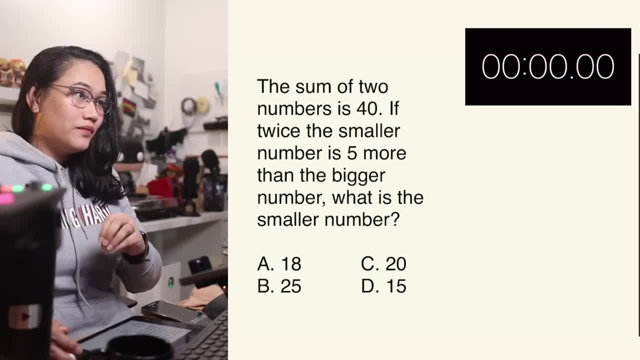 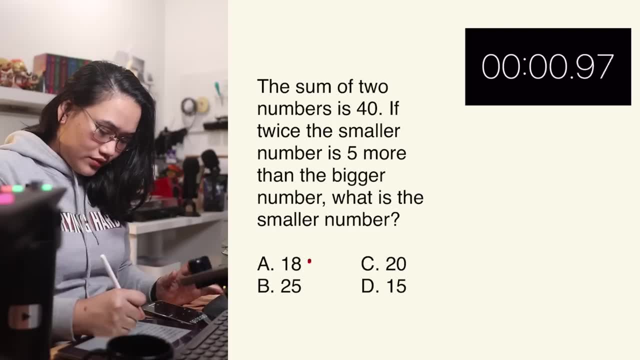 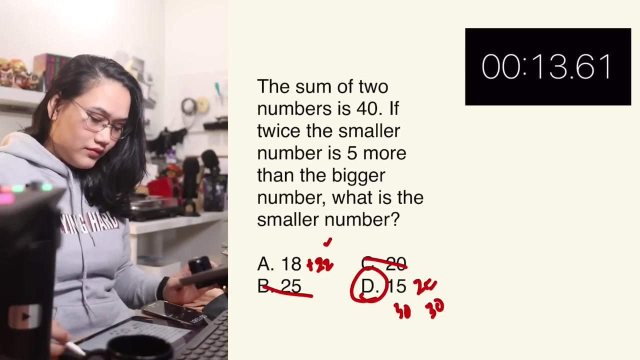 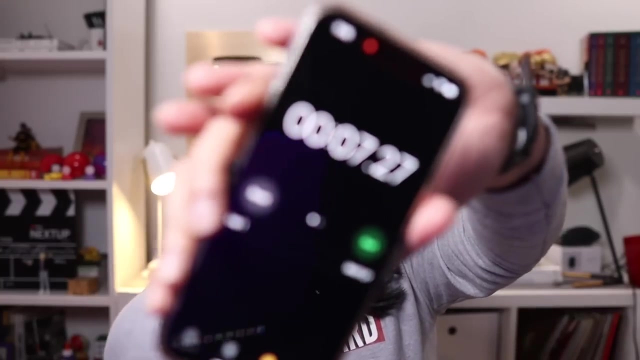 madali ka nang magtatanggal ng mga hindi pwedeng maging sagot. Now I'll show you how to do it And of course we'll time ourselves. So it took me 7 and some change seconds. na anong ginawa ko lang doon? 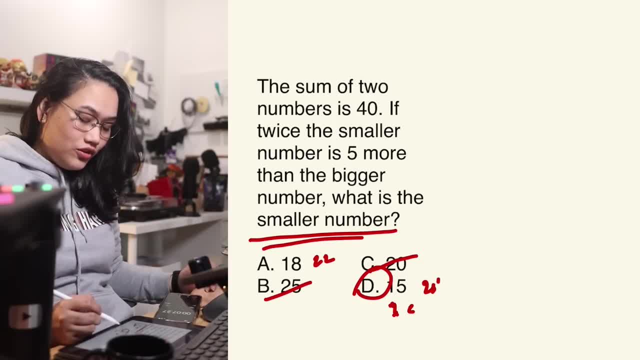 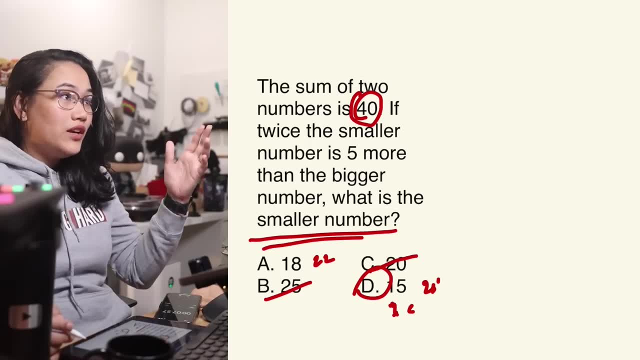 Dito, ako lang. ang hinahanap ay smaller number. So ibig sabihin nun, yung kapares niya or whatever is the number na idadagdag mo para maging 40, yung sum needs to be bigger. 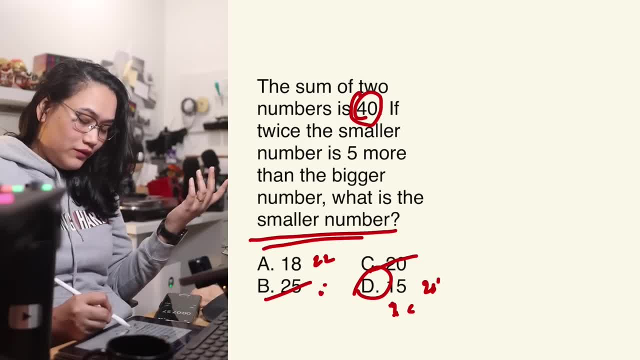 Hindi na pwedeng 25, kasi ang kapares niya to form 40 would be 15, which makes this the bigger number. Hindi na siya pwedeng maging smaller number. Hindi rin pwedeng 20, kasi pantay na sila. 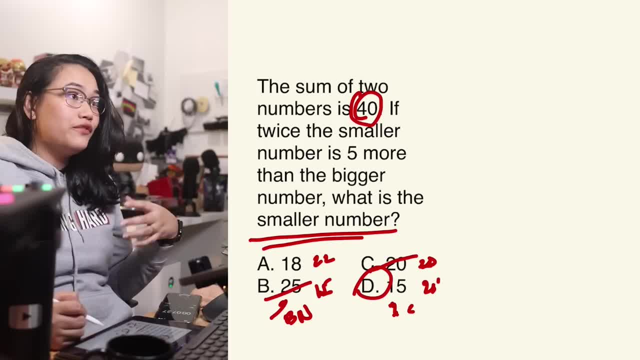 So wala nang bigger or smaller number, So it's either 18 or 15.. Now, just by looking at it, dahil alam natin twice: the smaller number is equal to 5 more than the bigger number. 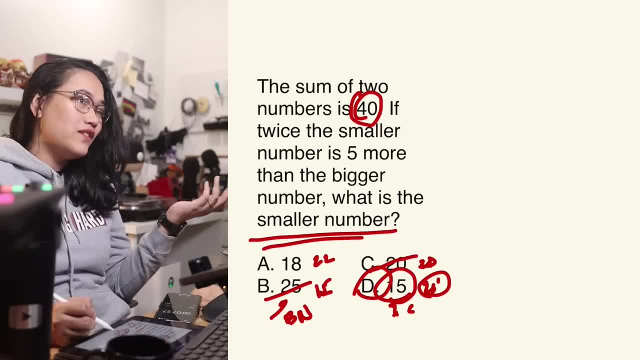 Tinayimsto ko lang in my head, yung 15, 30,, 25 plus 5 is 30.. Sagot na agad tayo. So anong preference ko kapag ako yung nage-exam? 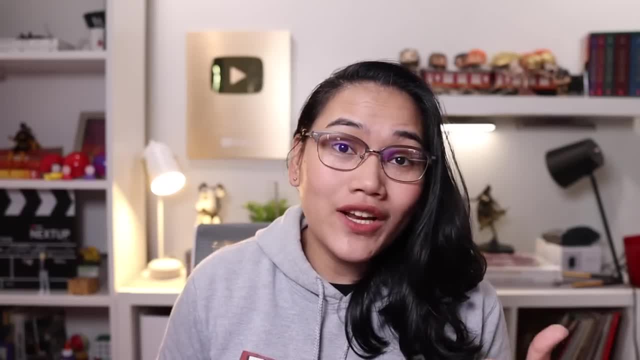 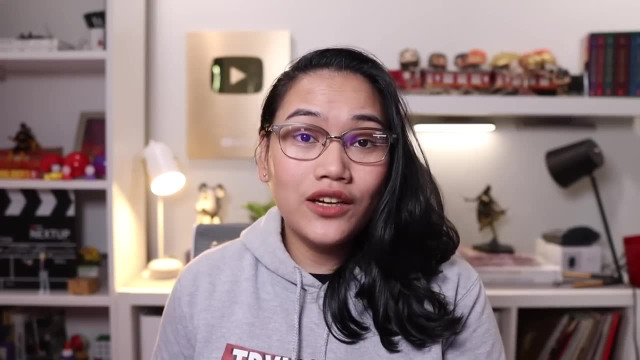 Sa totoo lang, ginagawa ko is number one: elimination agad. Kasi kung mag-e-eliminate ka na at nabawasan na yung mga options na pinagpipilian mo, kung magka-trial and error ka man, kaunti na lang yung susubukan mo. 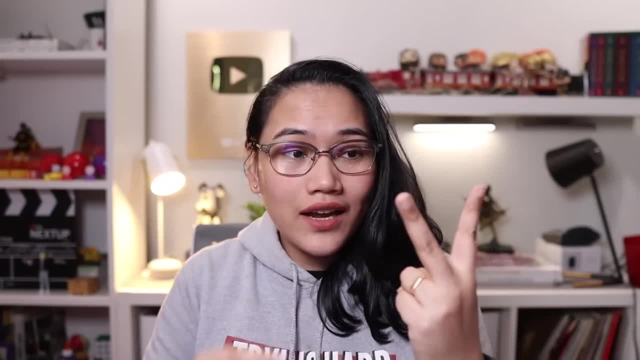 And, using common sense, pwede mo nang sabihin na kung dalawa na lang ang natitira at sinubukan mo yung isa, kahit hindi mo i-check itong isa, siya na agad yung sagot. 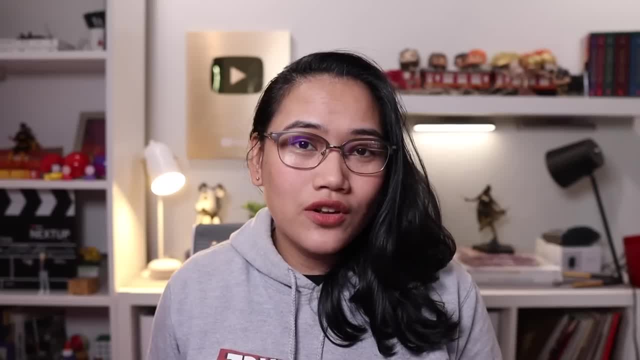 Which saves you time. i-shade mo na agad. Now, hindi ba ako nagsosolve pagdating sa exam? Well, kung kailangan, isosolve ko siya, Pero dahil nga nagmamadali tayo, ang lagi kong iniisip is: 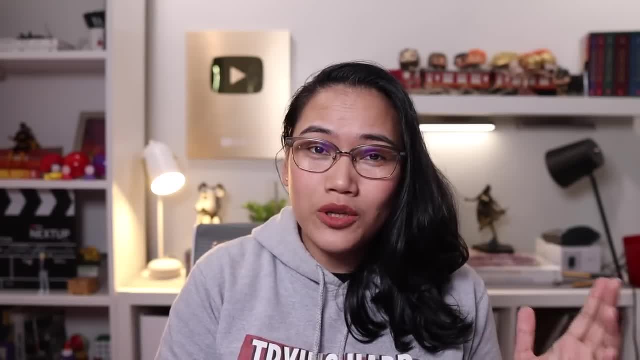 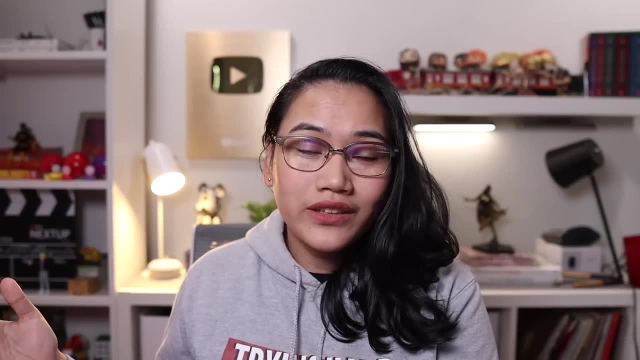 is it worth it to solve this entire equation from top to bottom, Or hulaan ko na lang tapos maghanap ako naman sa dadaling mga questions doon sa ibang parts ng test na pwede kong sagotan ng mabilis. 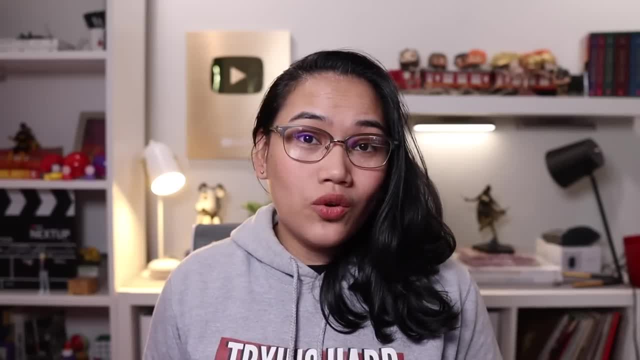 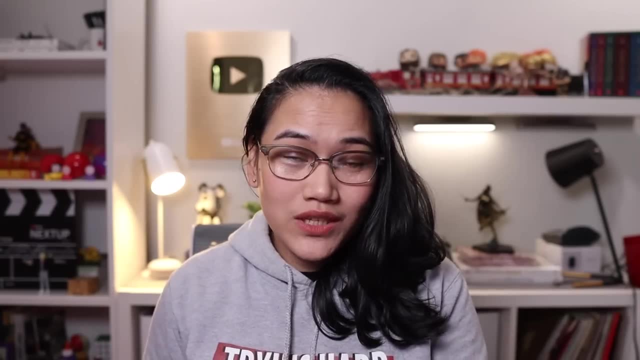 Common misconception ng test takers ang isipin na ang sinusukat dito ay pure knowledge, when in fact wisdom really comes into play, By definition ng knowledge is whatever you know. Wisdom is what you do with what you know. 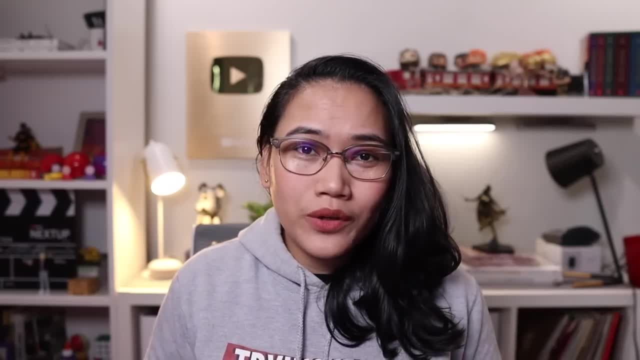 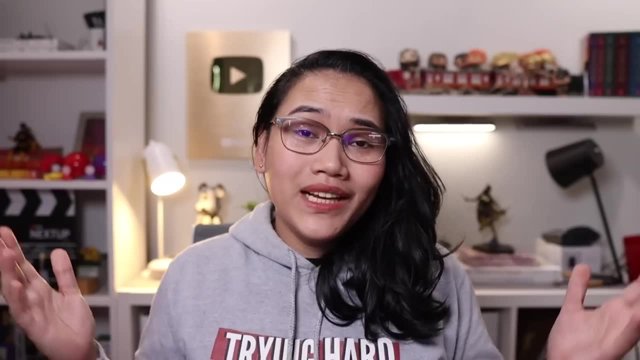 Yung decision making ba Yung weighing ng options kung ano yung mas worth it. Yung pag-discarte para makasagot ng mas marami at makakuha ng mas maraming tamang sagot. But again, this is just a study hack video that I made. 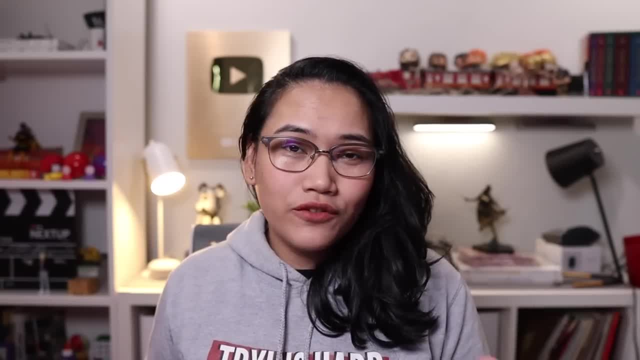 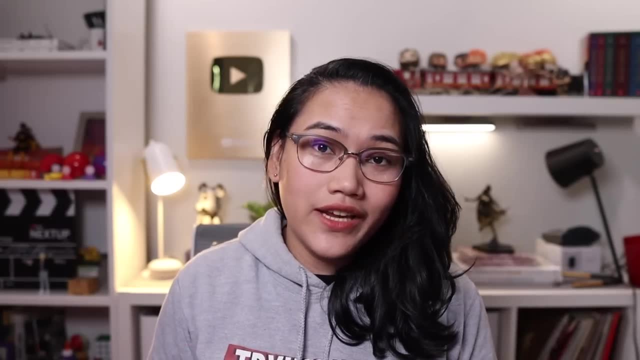 And sa lahat ng ito, ang key is to practice and encounter different types of questions. figure out, usually, kung gaano katagal kang nakakasagot, and in order for you to master all of these techniques, you really have to keep practicing by answering questions. 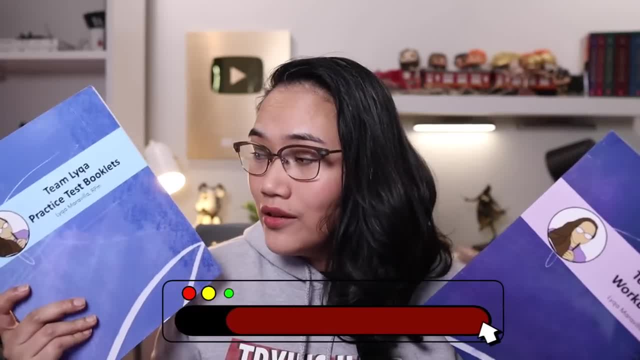 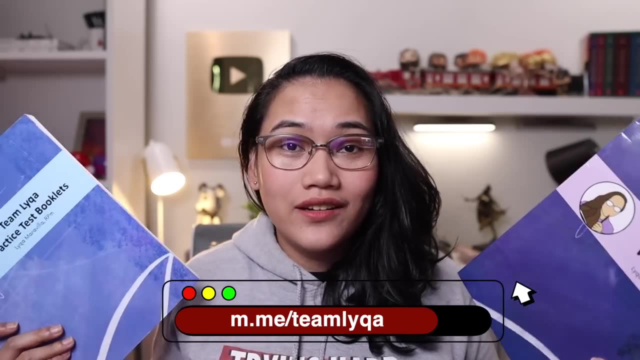 Again, if you're taking tests, we do have our practice test booklets and the workbook available right now. Kaka-restock lang namin, So if you're interested, go ahead and check out yung ating Facebook page, mmeteamlaika. 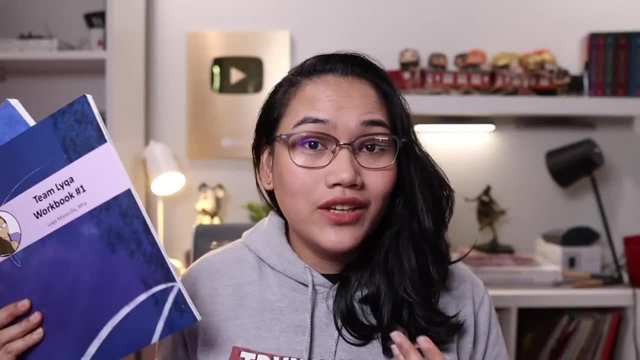 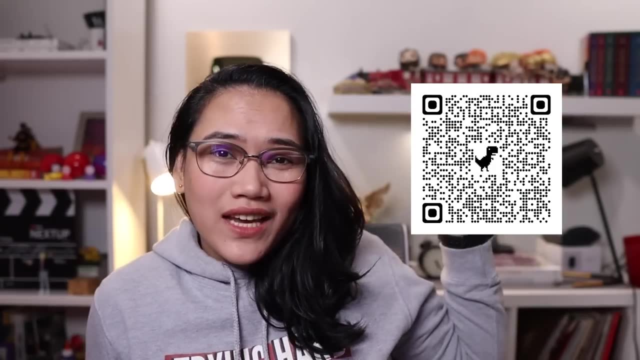 Lang yan sa inyong search bar. Message us on the page so you can learn how to get yours Nakuwala namang budget. okay lang yan. I actually included a free math diagnostic type of test right here And nakalink mo siya sa baba that you can take for free. 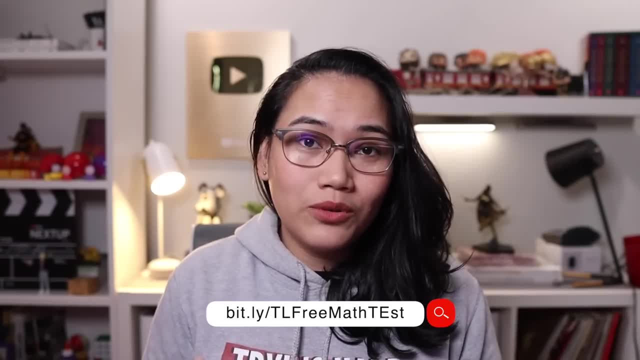 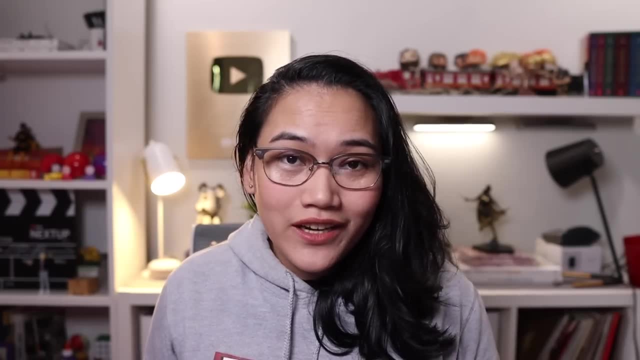 And may links din yan to the relevant lessons para matutuhan ninyo yung mga konsepto para dyan. So parang pabonus ko na rin sa inyo yan. But again, this is just my video, my opinion, my mini experiment right here. 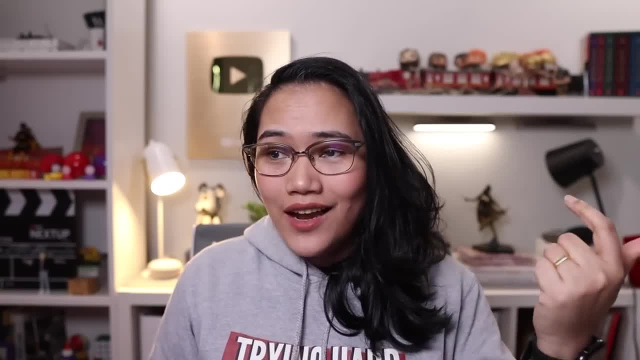 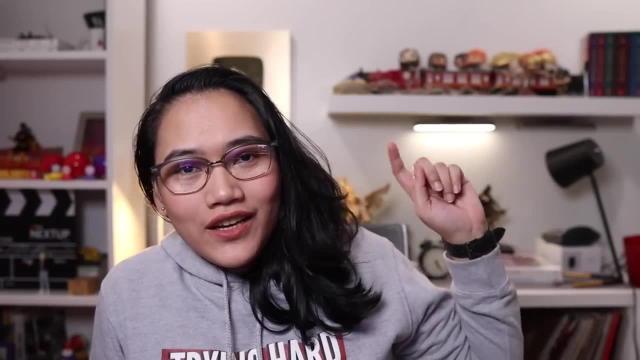 If you want more study hacks, videos, including what to eat, how to get better sleep or how to train yourself na makatulog, dahil importante yan, lalo na kung malapit ng examen ninyo, you can click right here dito sa taas sa i-button. 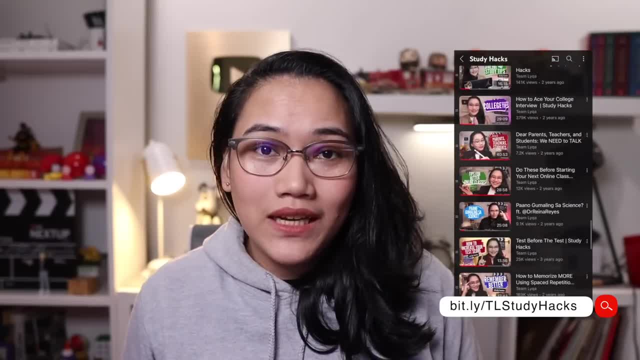 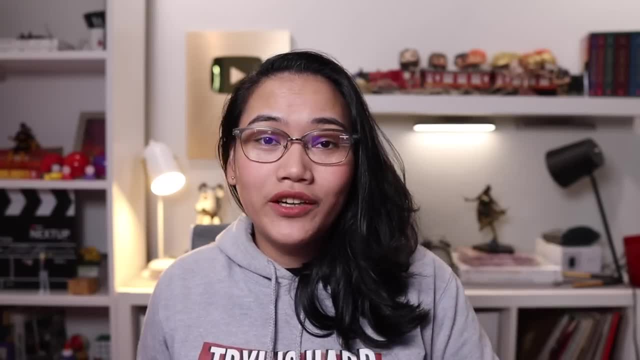 or find yung ating links sa ating study hacks playlist here and sa baba. Okay, Don't forget to subs. Don't forget to subscribe, lalo na if you're preparing to take a test, and for more educational content, As we always say sa channel neto.